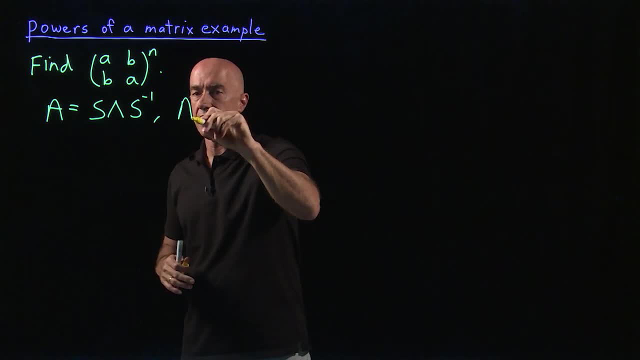 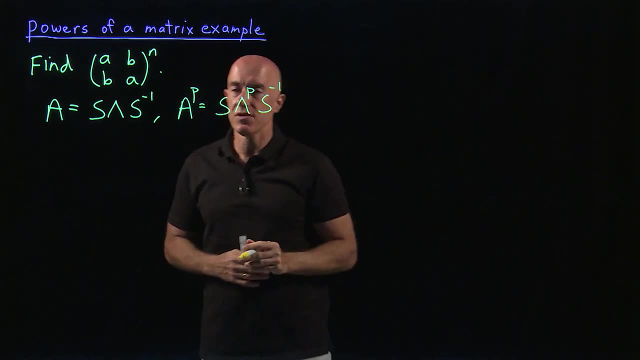 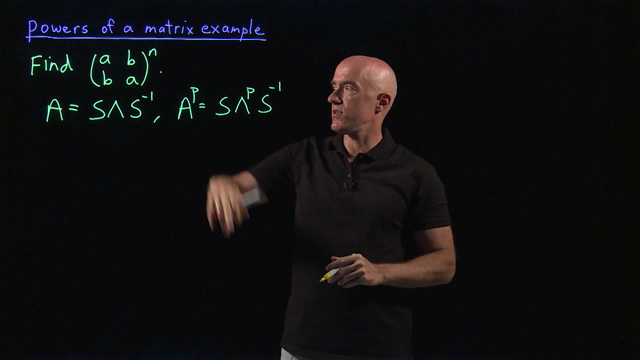 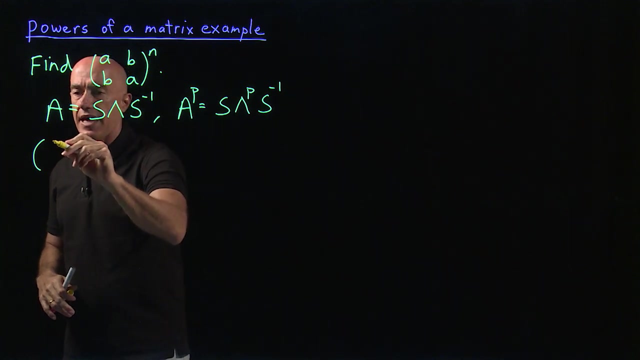 can then raise A to a large power. So A to the P then is equal to S lambda to the P times S inverse. Okay, So we know we've already computed S And S inverse for this matrix, So we'll use our result that ABEA is equal to one half. 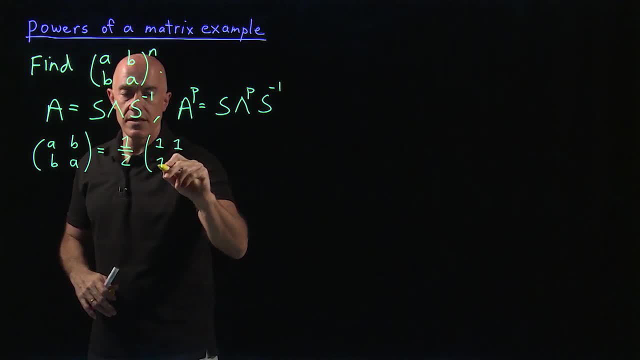 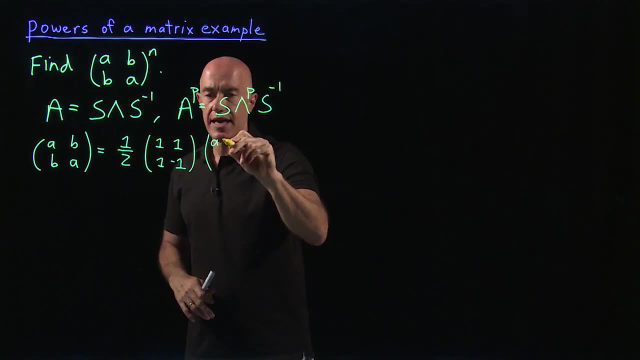 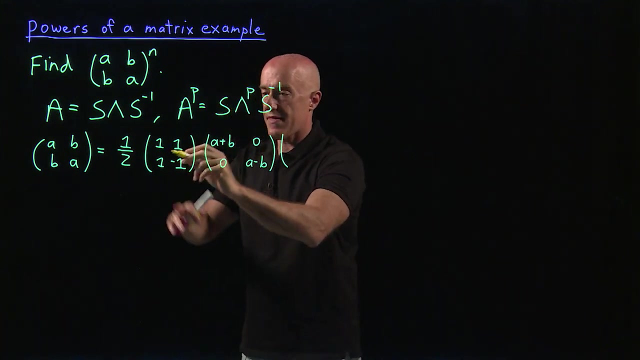 one, one, one minus one times the matrix of eigenvalues, which is A plus B, zero, zero, a minus e. And then the inverse matrix is the same as the matrix, So 1 over root, 2 times this matrix. 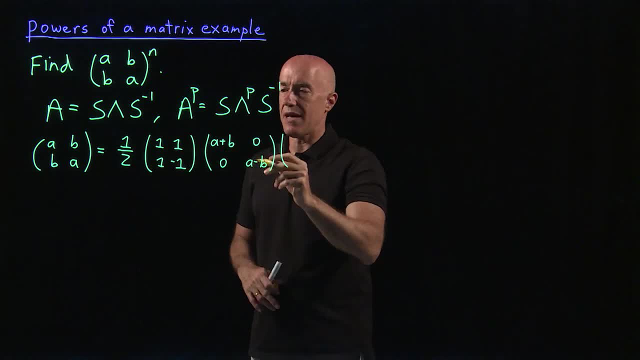 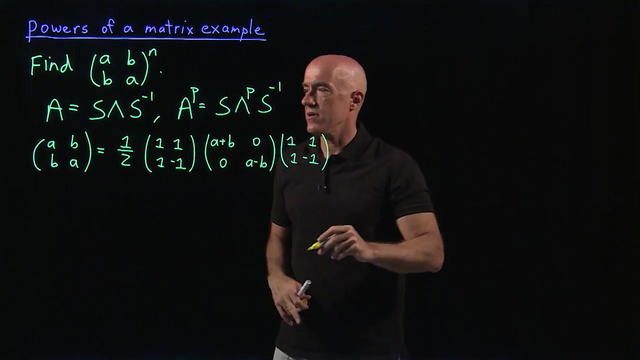 is s, And then 1 over root, 2 times the same matrix is s inverse. So this is 1, 1, 1, minus 1.. OK, We raise this to the nth power. So all we have to do to raise this matrix to the nth power. 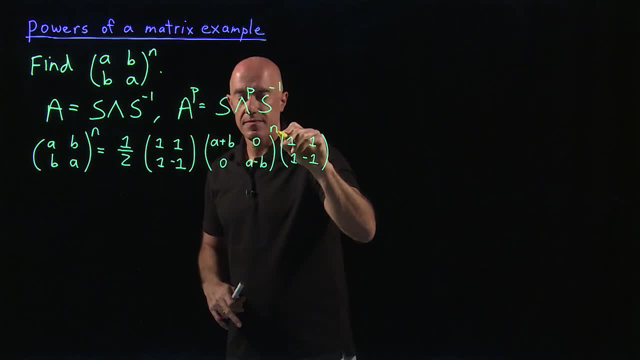 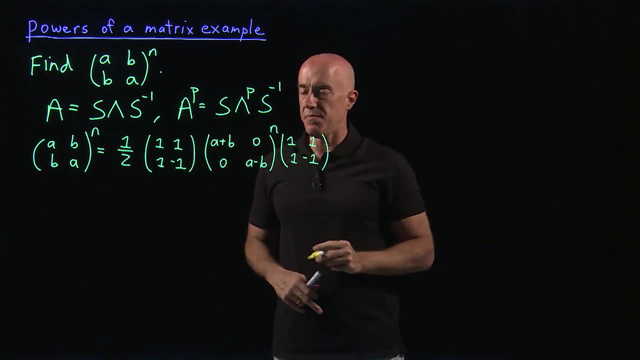 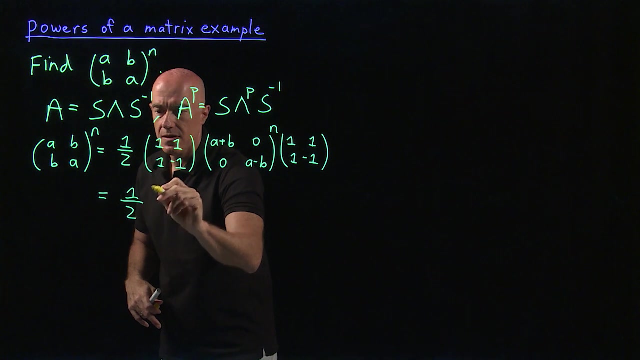 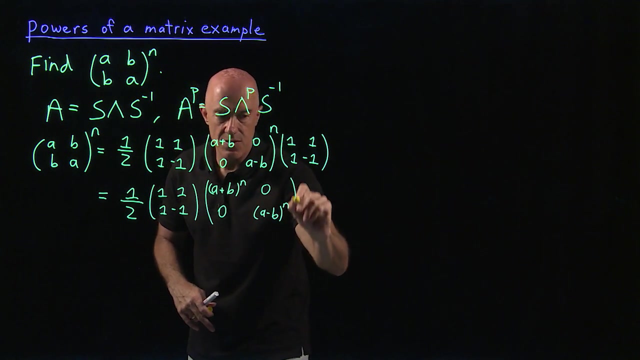 is raise this eigenvalue matrix to the nth power, which is the same thing as a plus b to the nth right. So this is simply 1 half 1, 1.. 1 minus 1 times a plus b to the nth power: 0, 0.. a minus b to the nth power, times 1, 1, 1, minus 1.. 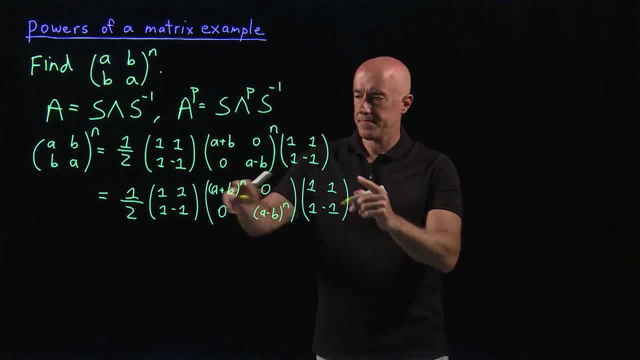 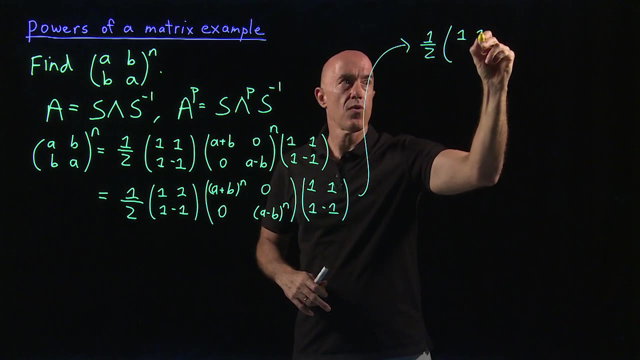 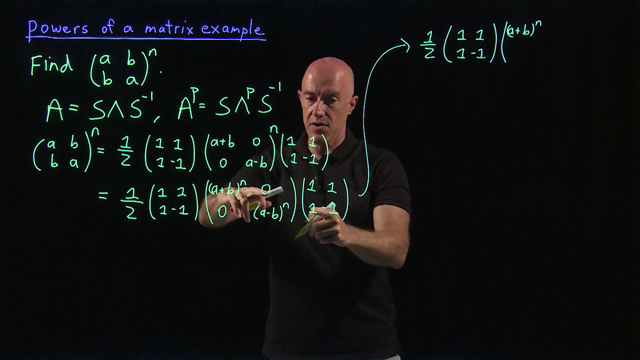 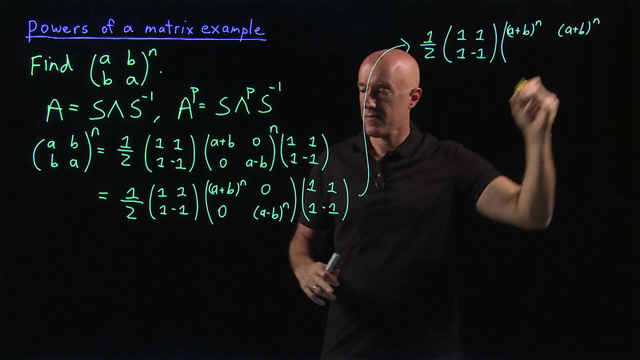 Now we just have two matrix multiplications to do, So we can go ahead and do them. So let's do this one first. So we have 1 half 1, 1, 1, minus 1.. And then a plus b to the nth plus 0.. a plus b to the nth plus 0. 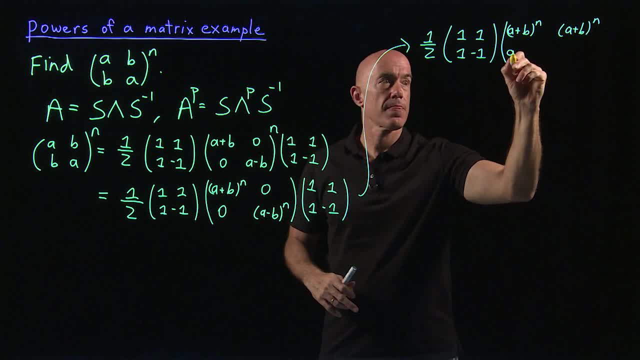 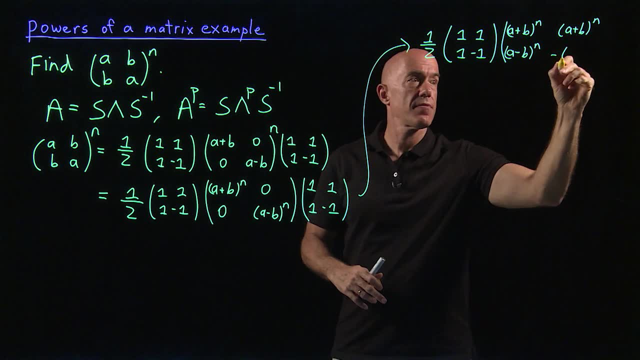 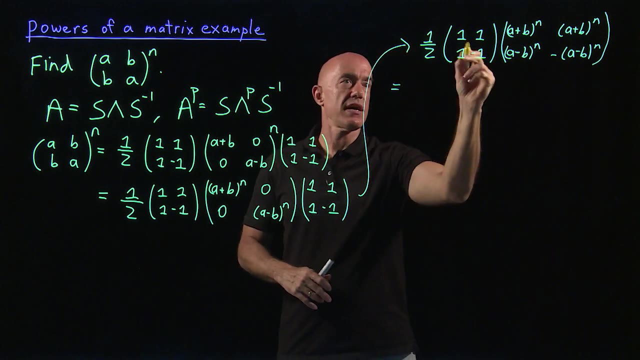 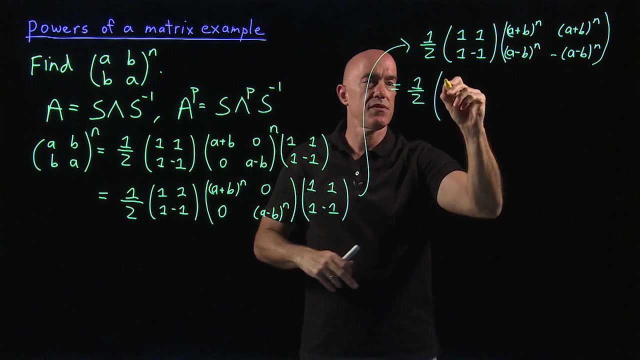 0.. a minus b to the nth And 0 minus a minus b to the nth. OK, One more matrix multiplication. So we have 1: half, And then we have a plus b to the nth, plus a minus b to the nth. 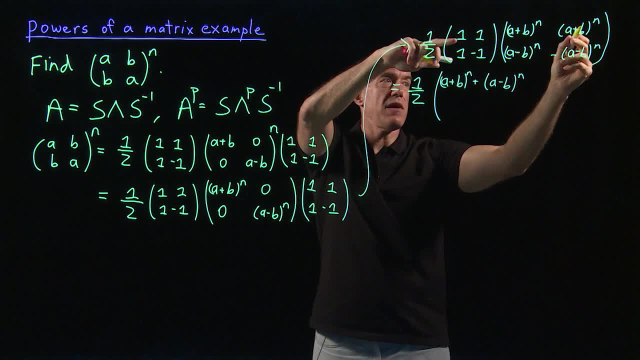 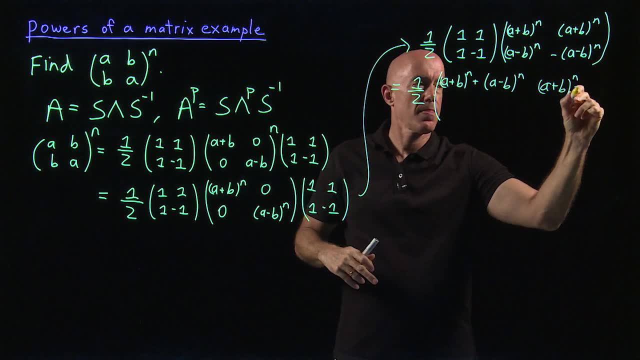 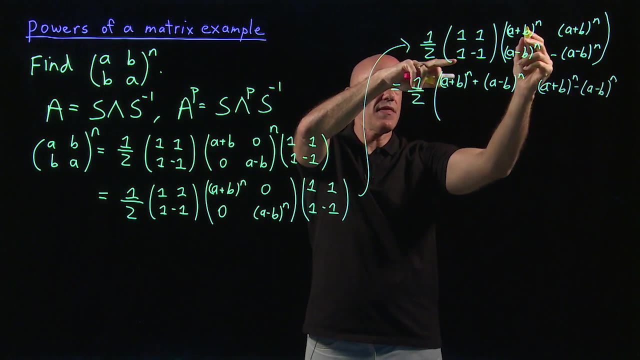 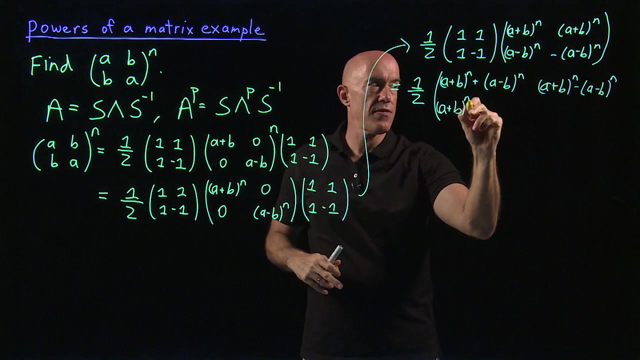 As the first element, And then we have a plus b to the nth, minus a minus b to the nth as the first row, second column, And then the same element here. So this is still symmetric matrix: a plus b to the nth, minus a minus b to the nth. 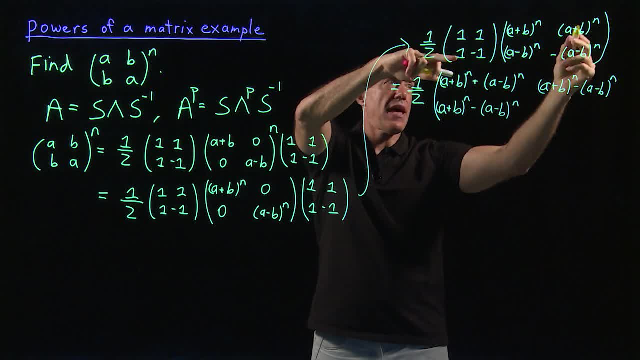 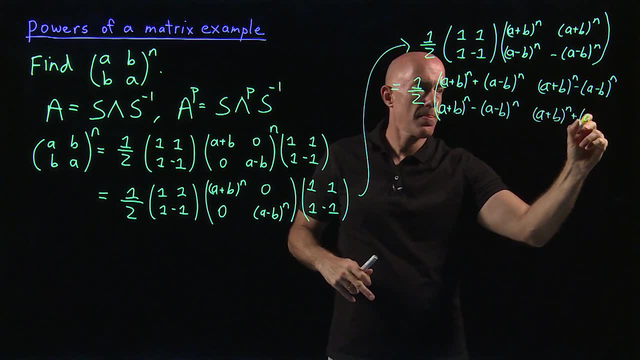 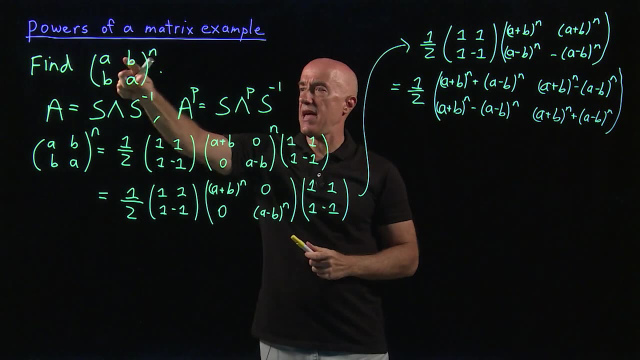 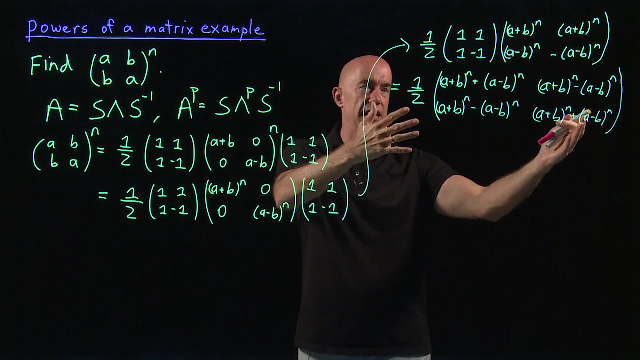 And then the last one is a plus b to the nth, plus a minus b to the nth. OK, So we've done. then found a b, b, a to the nth. is this 2 by 2 matrix, You can imagine: n is 1,000, something like this. 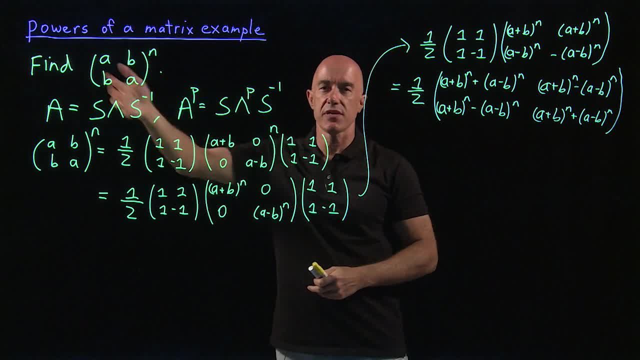 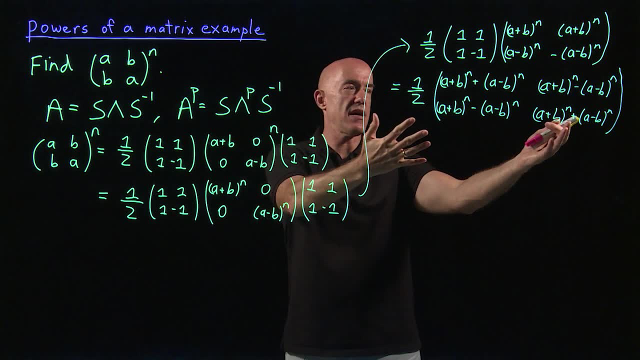 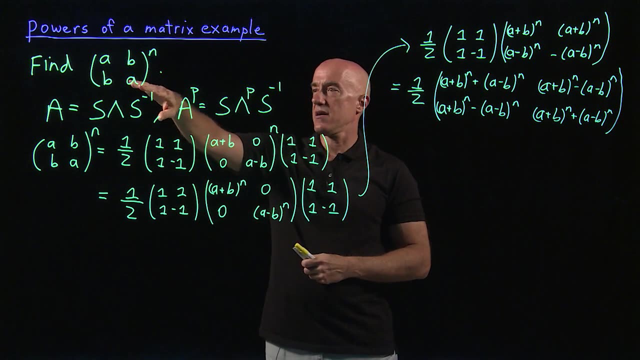 You're not going to sit here and compute this matrix times itself 1,000 times. But you can shortcut that process by first diagonalizing it And then you just have two multiplications, OK. So quick review To find a diagonalizable matrix raised to some integer power, some large power. 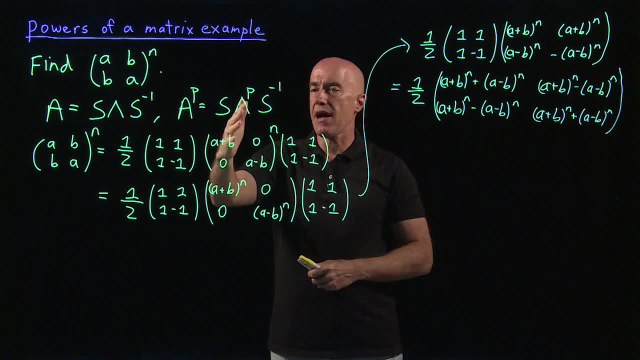 you diagonalize the matrix And then you raise it to a power is just the same thing as raising this diagonal matrix to a power. OK, So that's the diagonalized matrix raised to a power, which is simple to do. It's just the diagonal elements raised to that power. 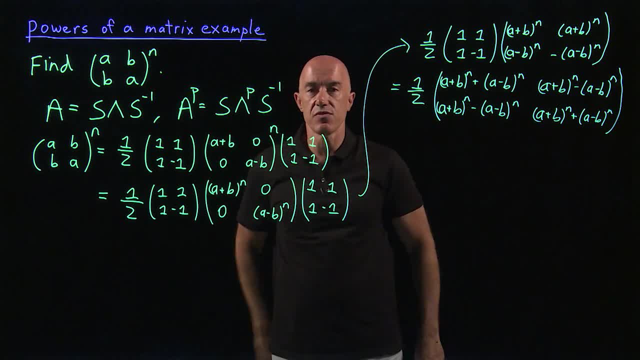 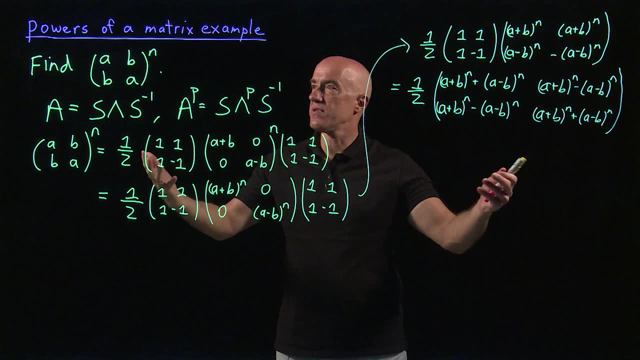 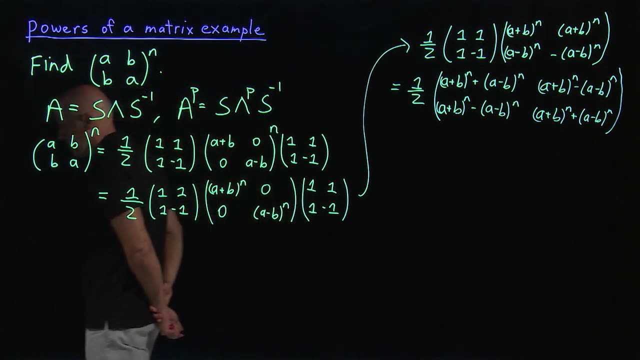 And then with two multiplications you can get the final result. I'm Jeff Chasnoff, Thanks for watching, And I hope you now understand the power of matrix diagonalization And how to design a matrix of a power equal to the power of a thank.